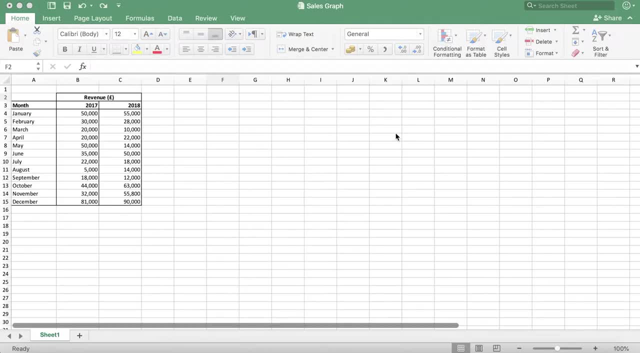 In this tutorial, I'm going to show you how you can compare revenue figures for two different years using a graph. For this example, I'll be creating a line graph to compare my data. However, you can also do this using a scatter or bar graph. 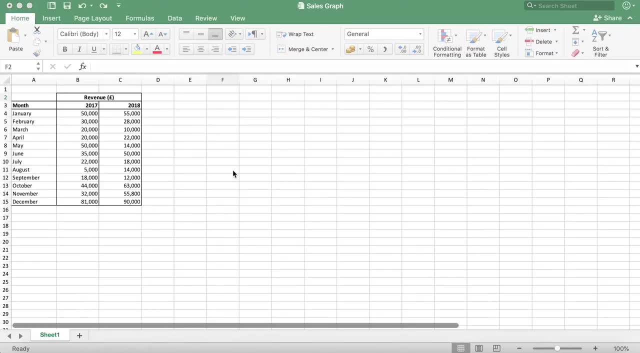 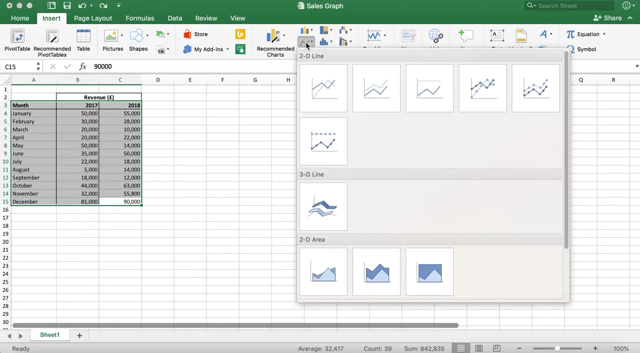 As you can see, I have already created my test data. I'll use this data to compare month by month revenue. Once you have set up your data, you need to select all the data as follows, and then click Insert, And then, from the Insert menu, I'm going to select the line graph and then select the graph I want to use. 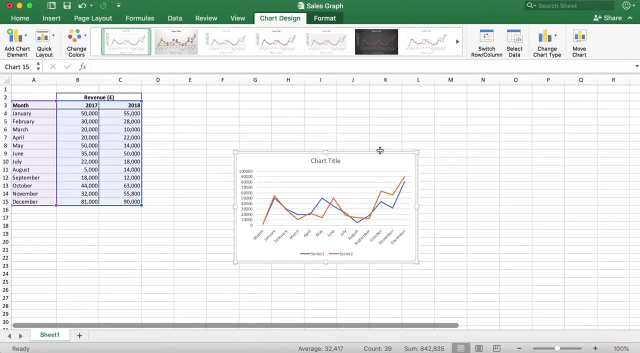 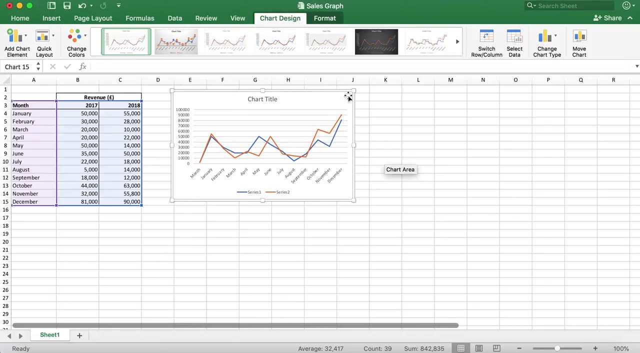 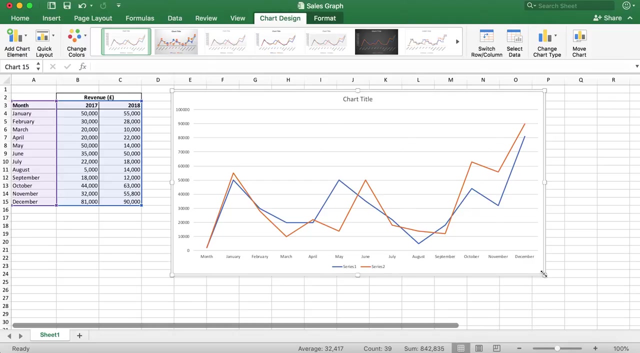 Now that the graph has been automatically generated, we just need to format it to suit our preference. I'm done. Now I'm going to move it to the top and resize it. To resize it, you can click and hold on any of the small squares around the chart and drag it to the appropriate size. 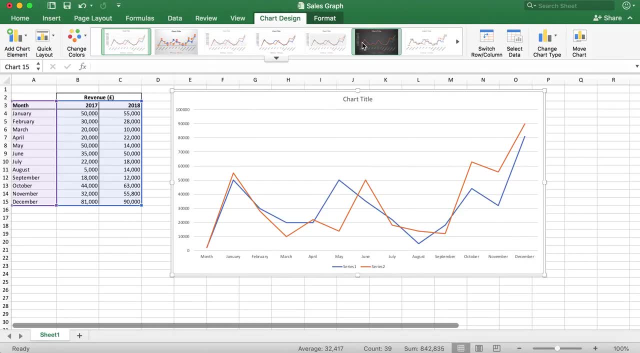 You can also use various options in the chart design to format it further. Now I'm going to give the chart a title. You can do this by simply clicking on Chart Title and renaming it. If you do not have a default chart title, you can add this by clicking on Add Chart Element, Chart Title and Above Chart. 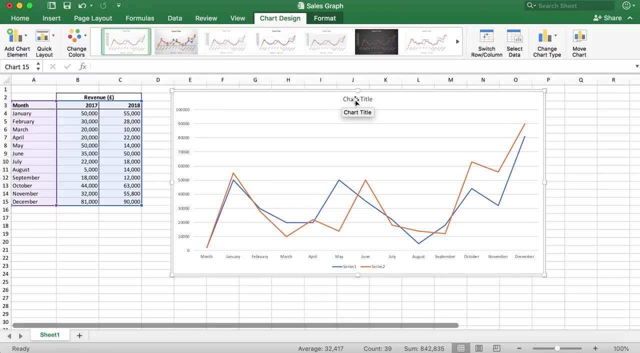 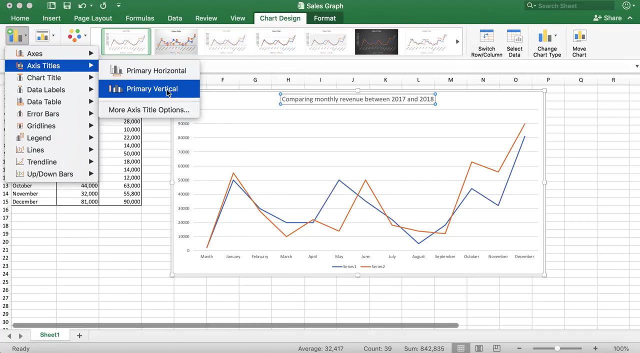 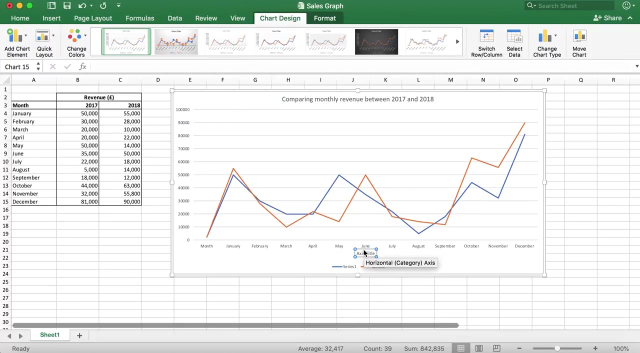 I'm going to call this chart Comparing Monthly Revenue between 2017 and 2018.. Now I'm also going to add an Axis Titles by clicking on Add Chart. Element: Axis Title: Primary, Horizontal or Primary Vertical. I'm going to call the Horizontal Axis Month and Vertical Axis Revenue.